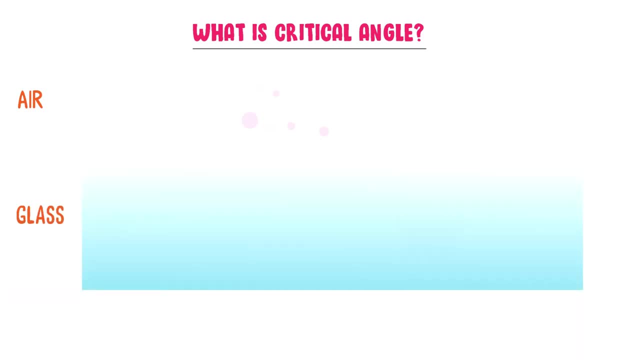 incidence and this is the angle of refraction. For instance, if I make a new eye wave, it will not let its eyes move, whateverblock it might, so its eye balance will depend on the moment of mówią. limitationsmet This is known as two medium. 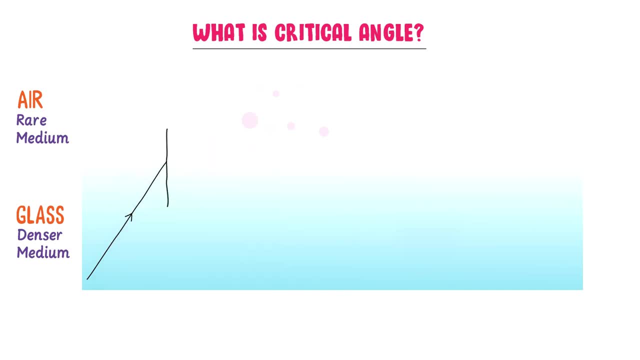 till these ends come nearer than the first shaper, As we know that optically, air is less denser medium and glass is more denser medium. let consider a light ray travelling from glass into the air. I draw normal line. Let this angle is 20 deg. Also, we have learnt that in the air, the refracted ray will bend away. 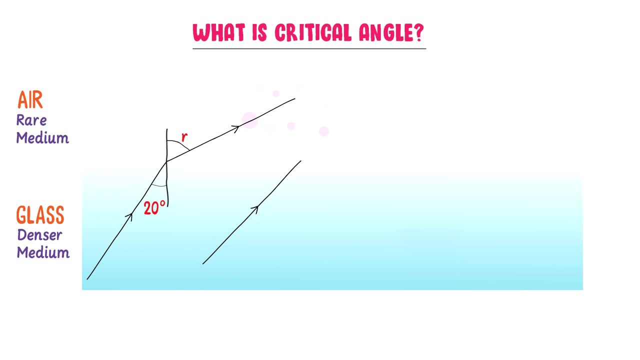 from the normal. Secondly, consider one another light ray. let this light ray also travel- strum讚, if grips- from another light ray, for example the left hand side Here, point tray- also travel from glass into the air. I draw the normal line. Let the angle of incidence 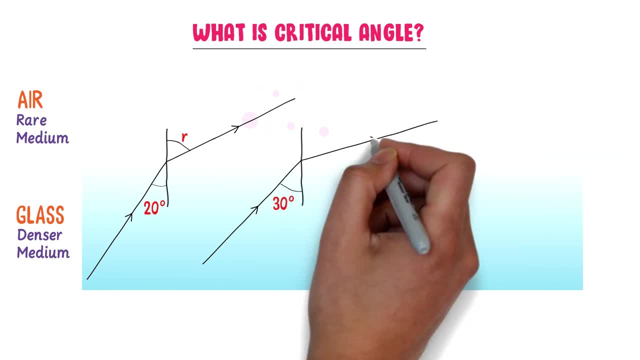 is 30 degree Now in the air, the refracted ray will bend away from the normal. Thirdly, consider one another incident tray Let it is travelling from the glass into the air. Let I draw the normal line Here. incident angle is 42 degree Now. in this case the 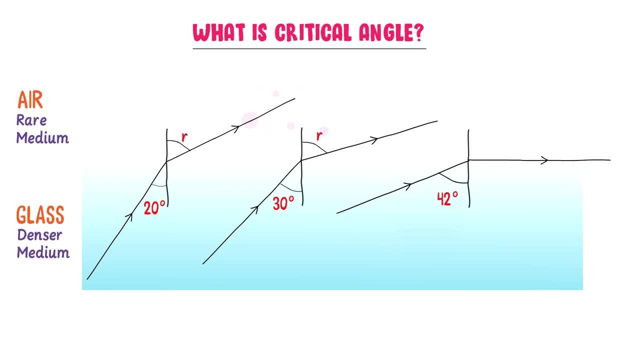 refracted ray will touch the boundary of glass and air and the refracted ray will be equal to 90 degree. So this incident angle of 42 degree is called critical angle, because for this angle the refracted ray is 90 degree. We can see that in the more denser medium. 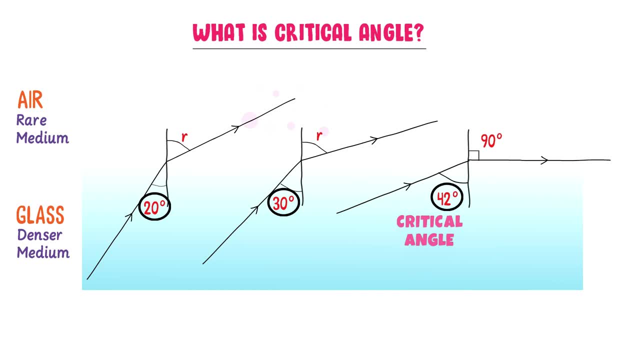 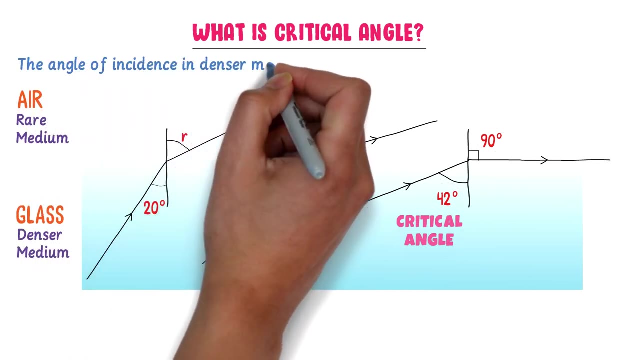 like glass. if we increase the angle of incidence, like 20 degree, then 30 degree, then 42 degree, the angle of refraction will be 90 degree. So we define critical angle as the angle of incidence and denser medium for which the 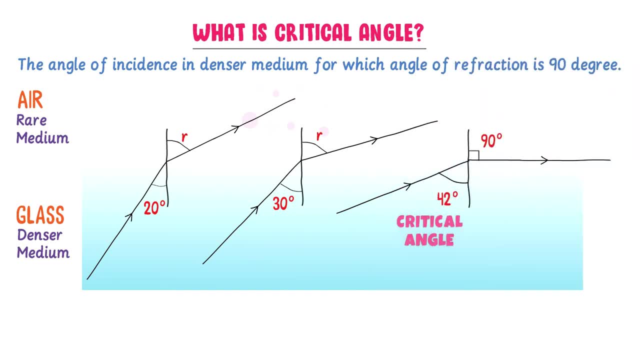 angle of refraction is 90 degree is called critical angle. Let me repeat this important point: The angle of incidence and denser medium, for which the angle of refraction is 90 degree, is called critical angle. So this 42 degree is the. 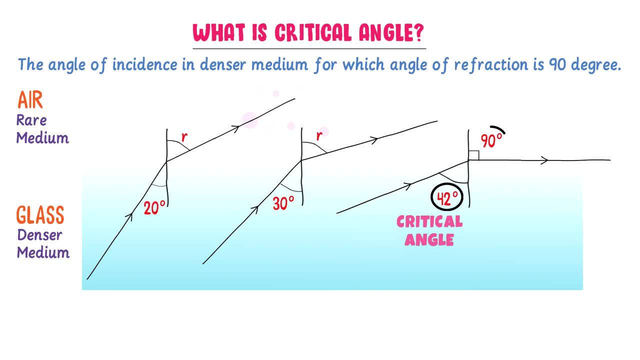 critical angle of glass. So this angle of refraction is 90 degree. is called critical angle of glass because the angle of refraction for this 42 degree is 90 degree. Note it down, these two important conditions of critical angle. Firstly, angle of incidence. 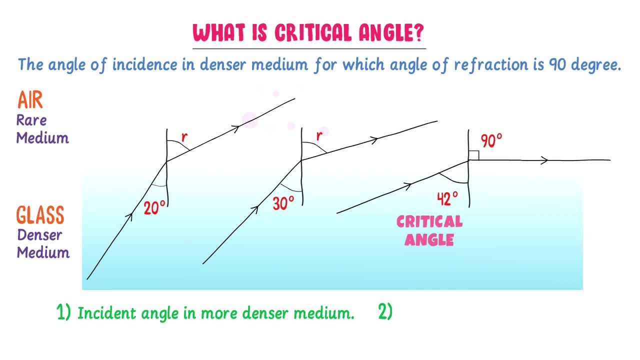 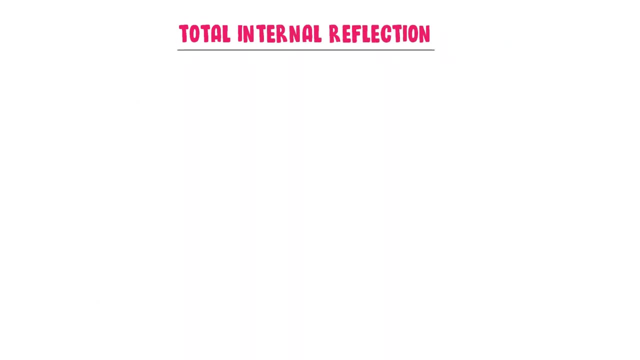 must be in more denser medium. Secondly, refracted angle in less denser medium must be equal to 90 degree. Thus note it down, all these important points. Now, what is total internal reflection? Again, consider two media like air and glass. Let a light ray is travelling from the more. 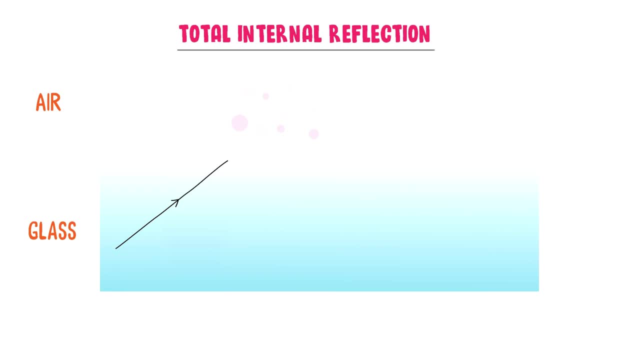 denser medium and to the less denser medium. Here I draw the normal line. Let the incidence angle is equal to 42 degree. We know that the critical angle of glass is 42 degree, So the refracted angle and the less denser medium will be equal to 90 degree. Now consider: 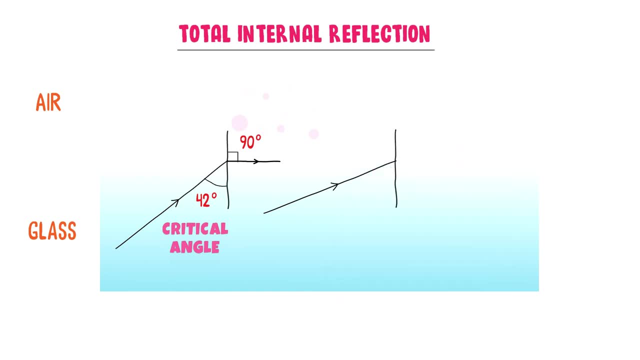 one another incident: ray- I draw the normal line Here. the incidence angle is equal to 43 degree. It means that 43 degree is greater than critical angle of glass. Let me repeat this important point: 43 degree is greater than critical angle of glass. Now, in this case, the total light will 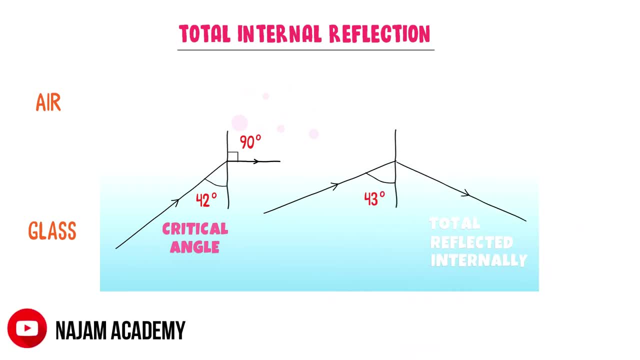 be reflected within the glass. Let me repeat it: The total light will be reflected in the glass. Here no reflection occurs. The total light is reflected internally. So we say that this is total internal reflection. Here we can apply all the laws of reflection. For example: 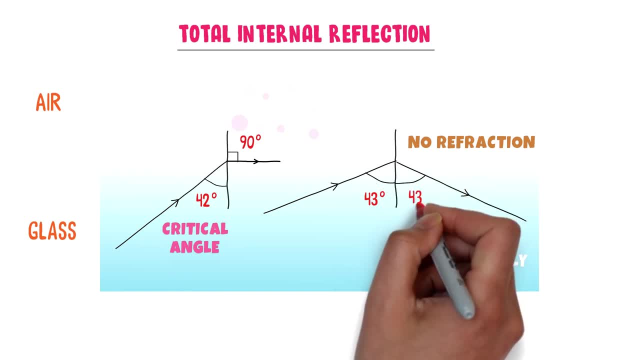 the incidence angle is 43 degree, So the angle of reflection is also 43 degree. So we say that this phenomena is called total internal reflection. Therefore we define total internal reflection. Let me repeat this again: Here no reflection occurs. The total light is reflected internally. 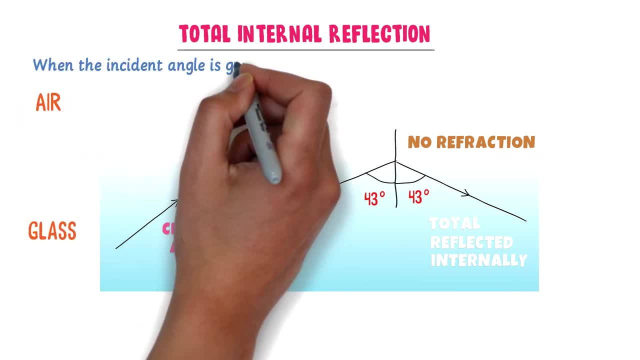 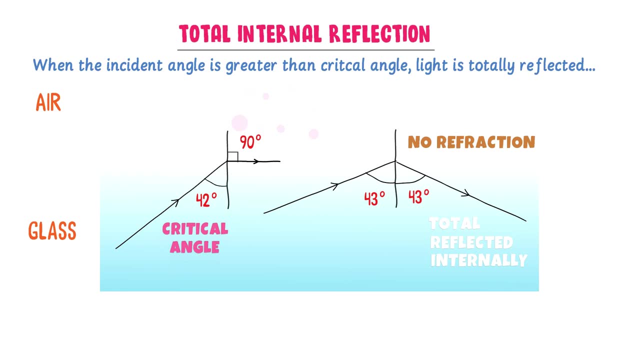 So we define total internal reflection as when the angle of incidence is greater than critical angle, light is totally reflected within the same medium. So we say that this is total internal reflection and this is not total internal reflection because here still light is reflected. Also noted down two important conditions of total internal reflection. Firstly, light.